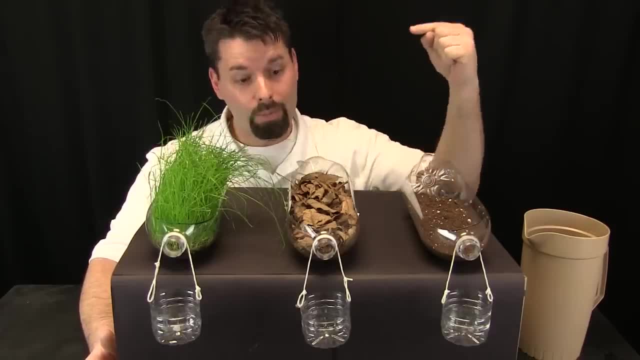 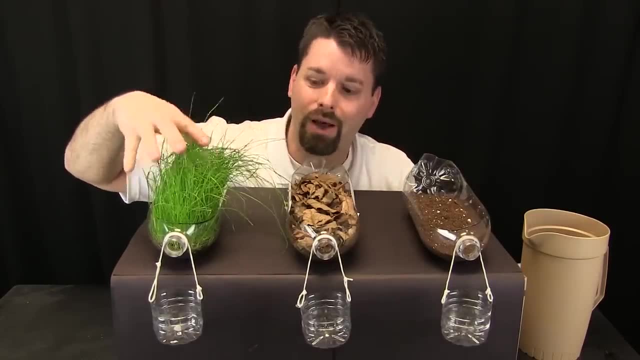 comes out into the cup, Will it be any different from the water we pour into this bottle as it comes into the cup, And will this one be any different when we pour water into this bottle and it comes out into this cup? So I am going to slowly pour water in, You are. 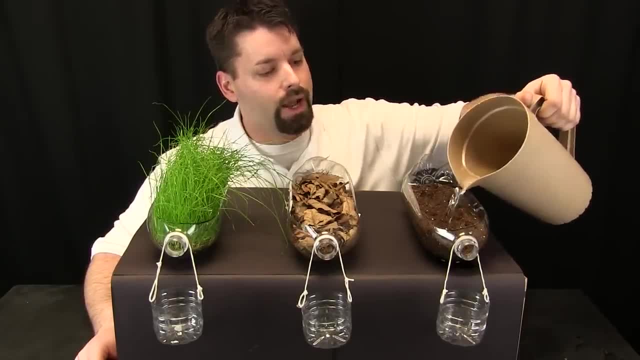 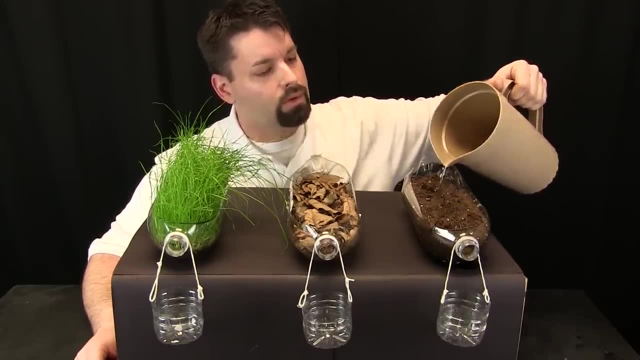 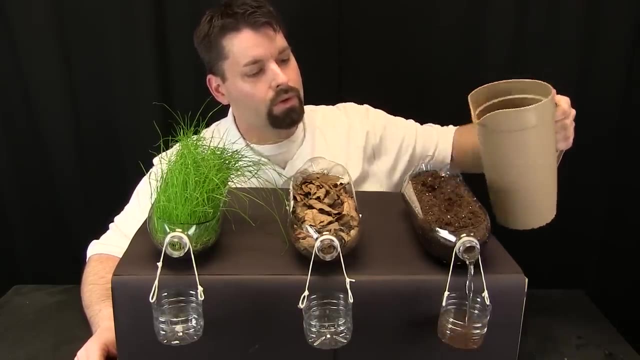 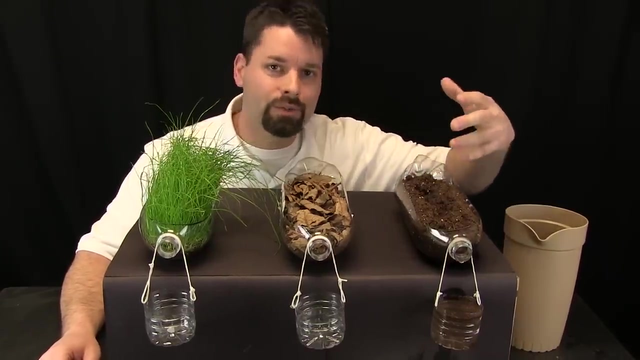 going to see the water level rise and we will see what happens with our soil. We will keep it coming, and now it is coming out. Take a look at the bottle we used to catch the water. What do you notice? It is cloudy. So why is it cloudy? That is because 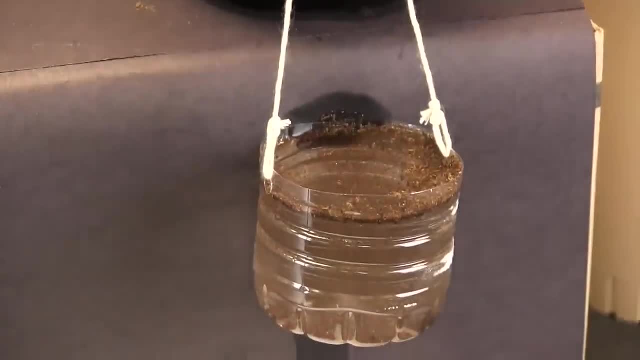 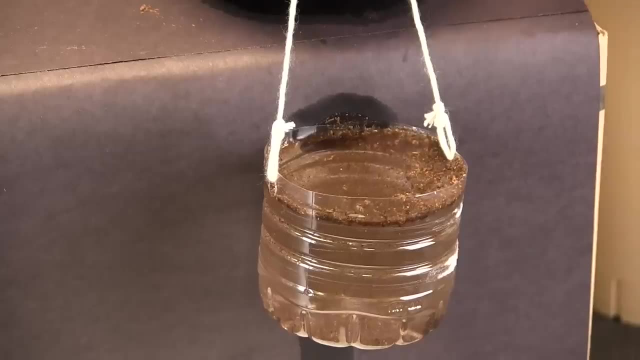 all the dirt and the soil from our bottle was washed into the cup. The water had the power to actually take the dirt and the soil with it and it is going to change the land With it. out of the bottle and into the cup. The water moved the soil, It shaped the soil. 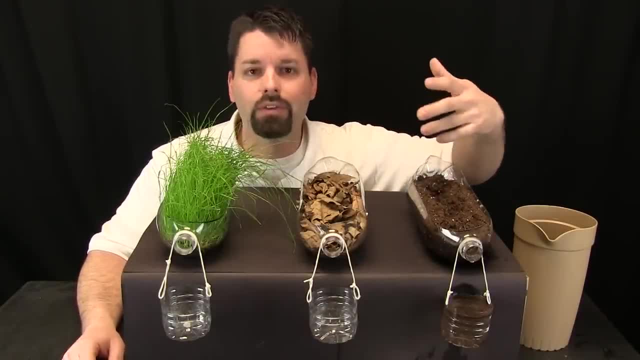 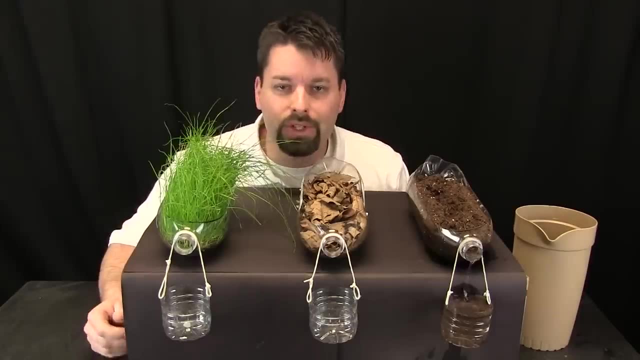 So now I am going to pour about the same amount of water into the next bottle. What do you think is going to happen? The water that we catch, will it be just as dirty? Will it be less dirty? Will we even be able to see a difference? Well, let us pour the water and 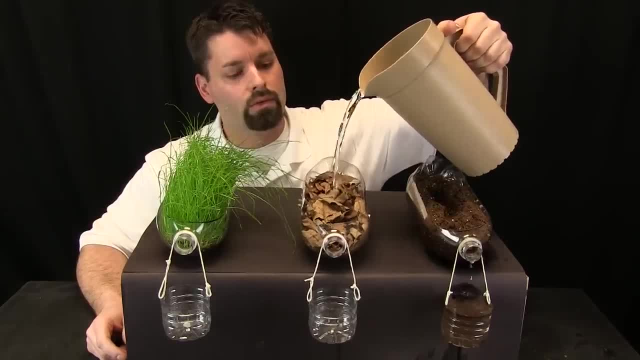 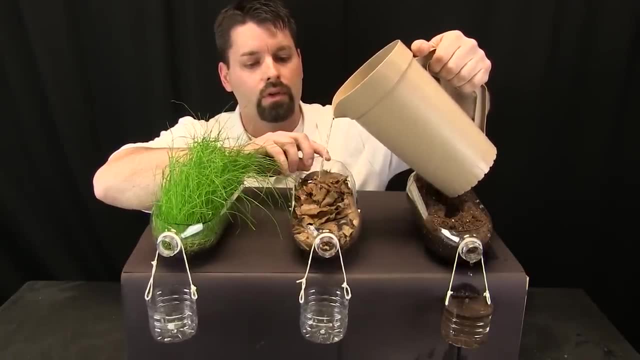 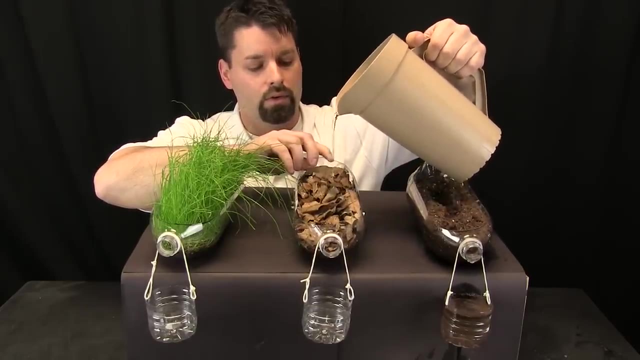 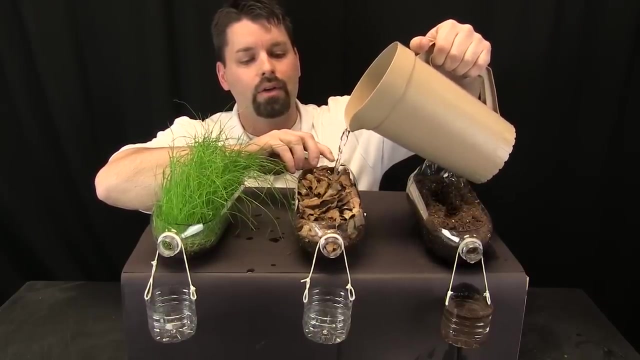 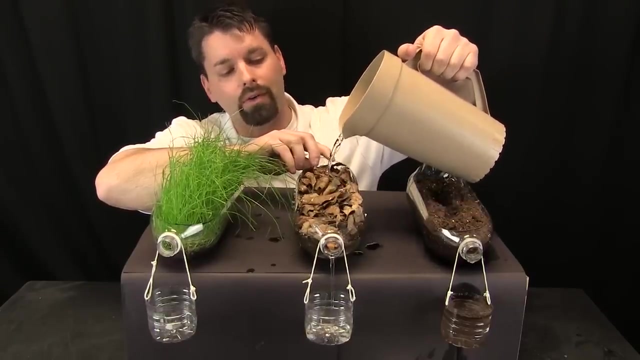 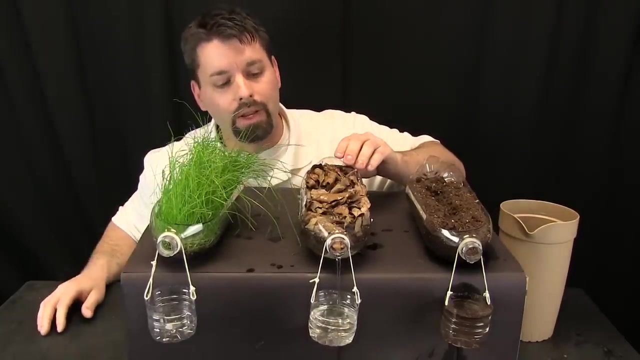 find out. Here we go. So I am pouring the water in, Making it rain, Adding water to our bottle. I can see the leaves floating to the top. Do we have any overflow? Yes, we do. Stop the rain and see what we have. So we have zoomed in so you can compare. 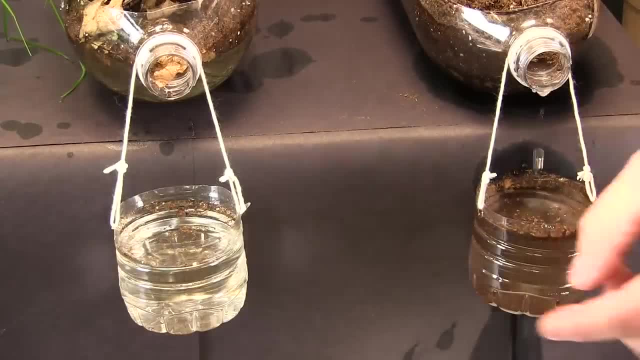 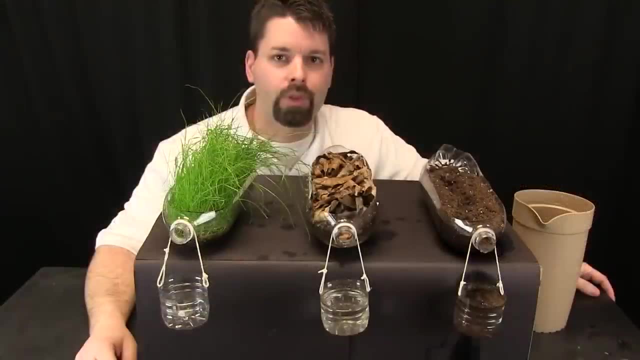 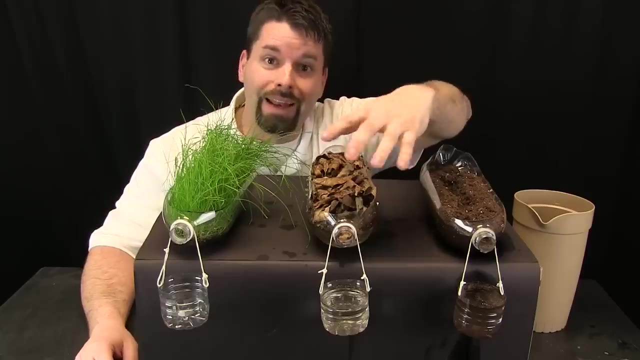 the two. This one has a lot of the soil in the container. This one just has a little bit of the particles, a little bit of the soil in that water. So why you think this container is a little bit cleaner. Well, what is different between the two? Well, this one. 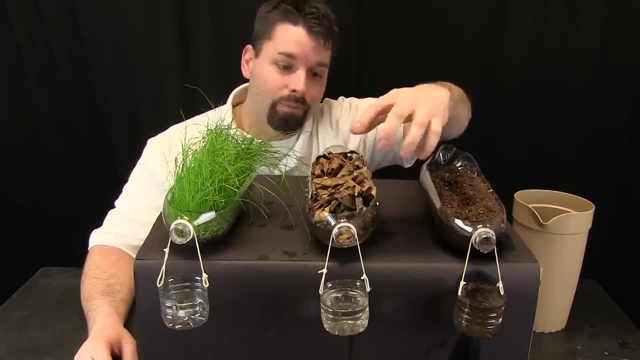 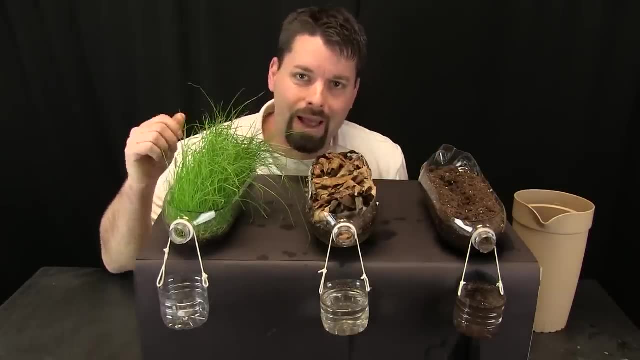 had leaves- dead leaves- on top, and I think most of these dead leaves helped protect the soil underneath from moving with the water. So what do you think is going to happen with our third container? We have plants growing in the soil. What is going? 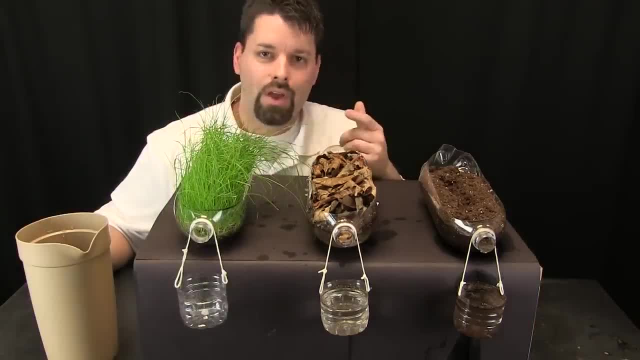 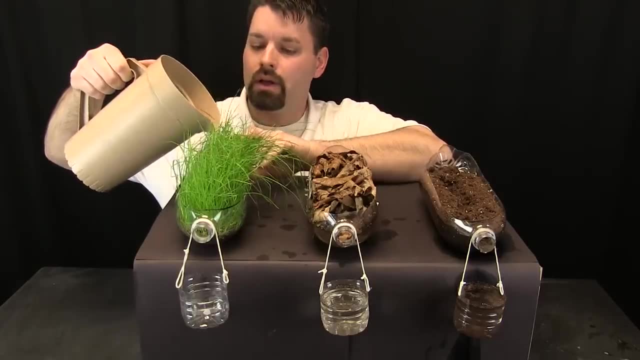 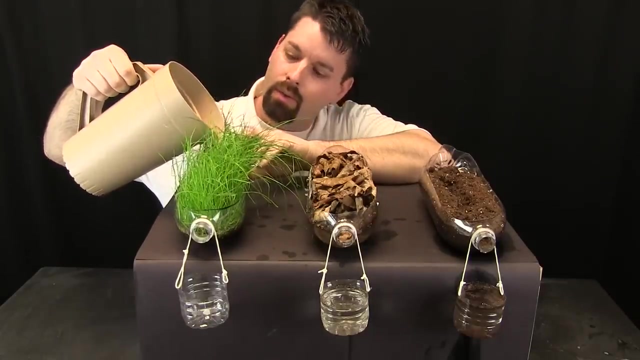 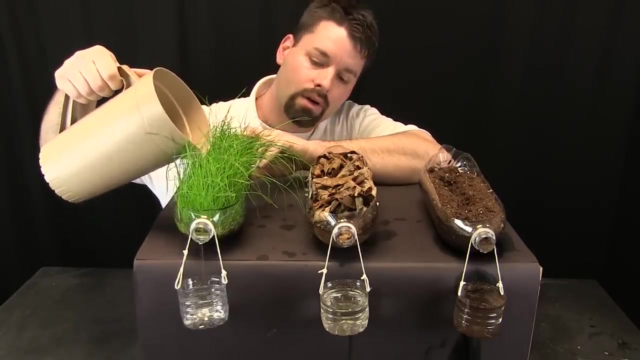 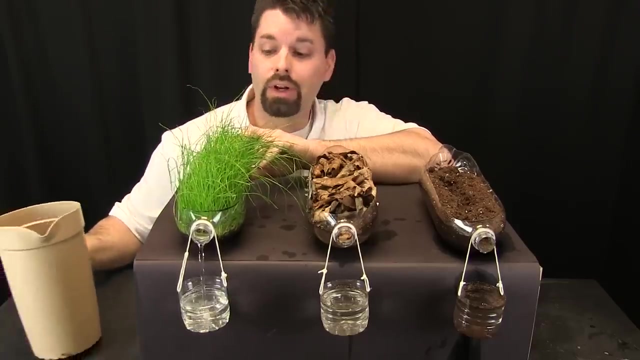 to happen when we add water and make it rain in this container. Alright, here we go. Let us add the water about the same amount. pouring the water in. What do you think is going to happen here? Add a little bit more, It is coming out. We are going to. 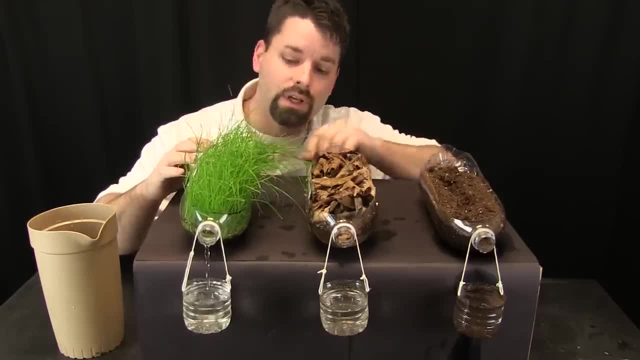 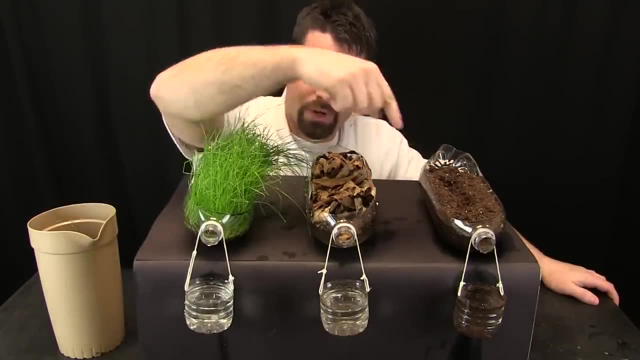 stop pouring and see if we can compare what we see coming out. The water coming out of this container looks a whole lot cleaner than this one and a little bit cleaner than this one. So the question is: why? Why is this water cleaner? I poured. 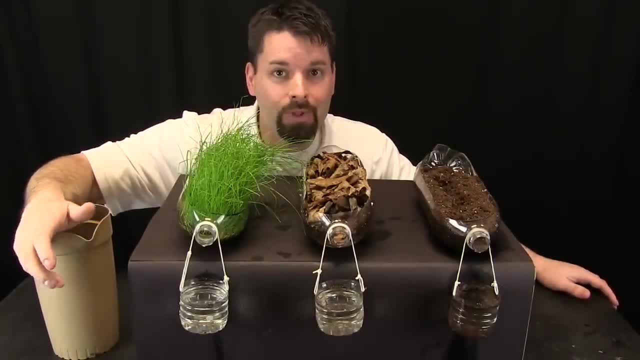 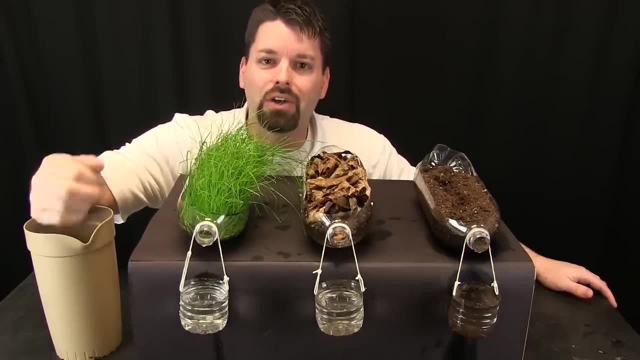 about the same amount of water out of this container. I poured about the same amount of water into each container of soil. This one looks really clean. Well, to answer the question why we have to zoom in and take a closer look at what, 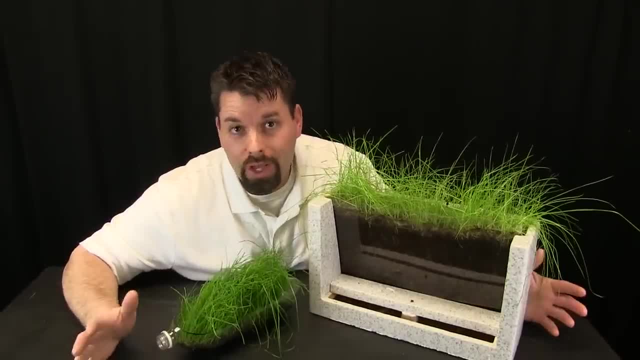 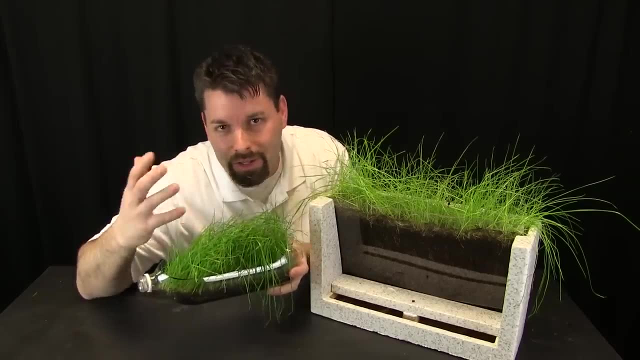 is really going on here. So now we are all set to take a closer look at why the water coming out of this bottle was so clean and clear compared to the others. To do that, I am going to actually lift these plants out of this bottle and let us 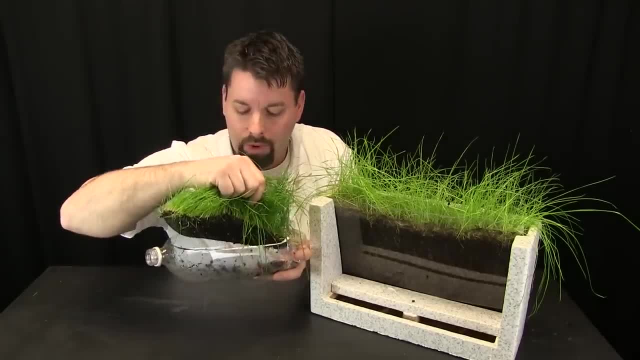 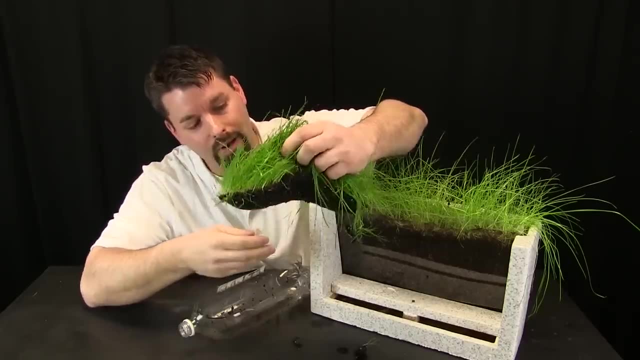 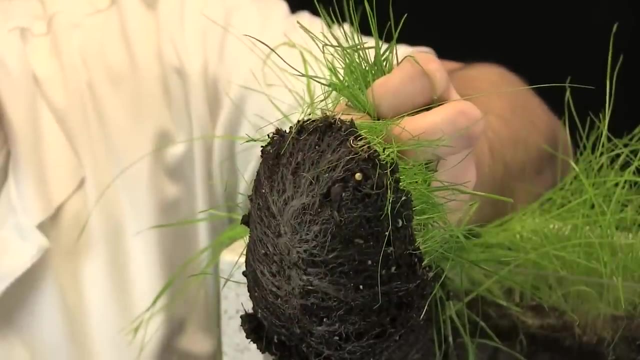 see what happens. Well, what I noticed right away is what comes along with all of the plants. Well, the soil is actually coming out too. When I flip it over, I think you will be able to see why. So we have zoomed in so we can see what is going on here. Why is this soil staying together? 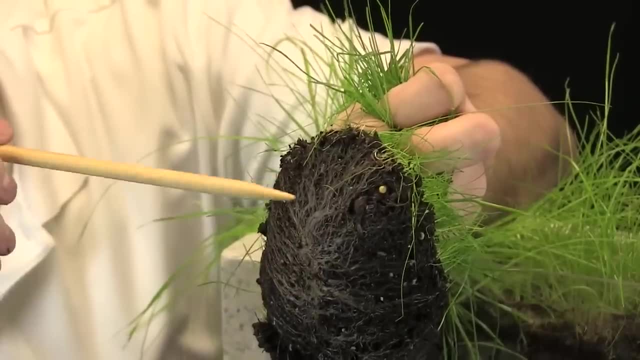 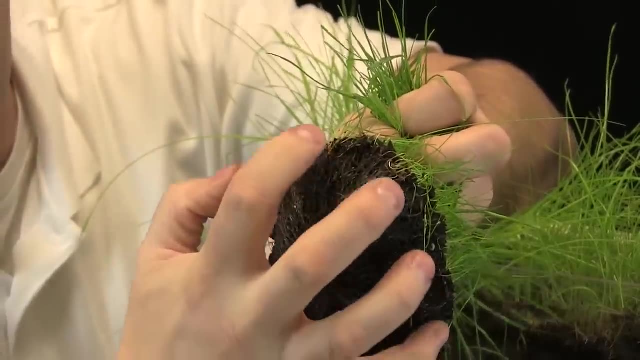 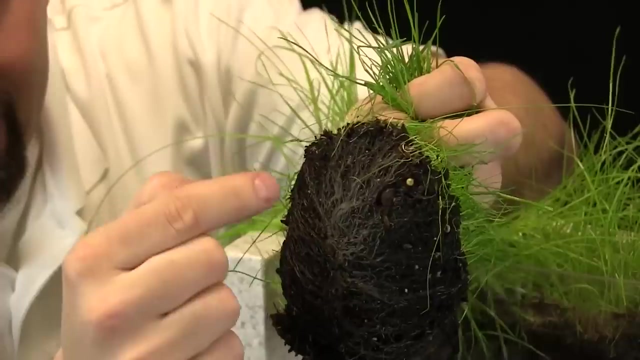 Why is it staying in place? Well, you can see, the roots from our plants grew into the soil and, almost like little fingers, those roots are holding the soil together. So when it rains, the roots keep the soil from washing away. The roots of the plant. that is what keeps the water from eroding. 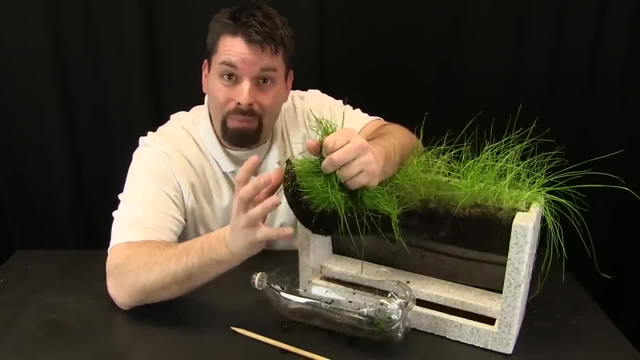 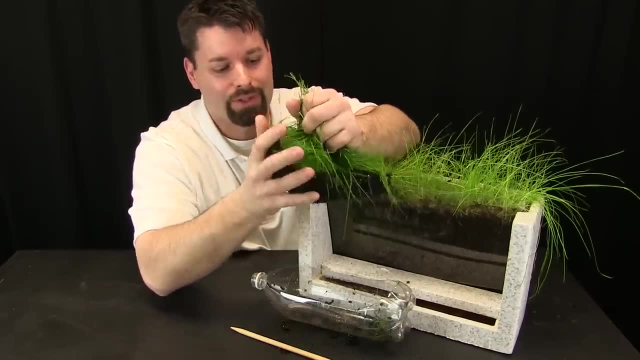 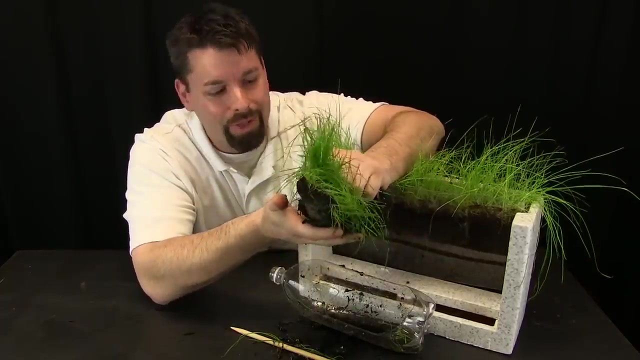 the soil. Besides holding the soil together and in place, roots do another amazing thing: To show you that I am going to squeeze this and I want you to watch what happens. Where did all that water come from? Well, that came from when we made it rain on our soil: The